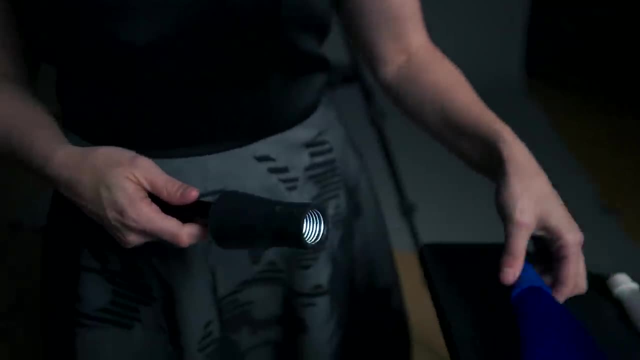 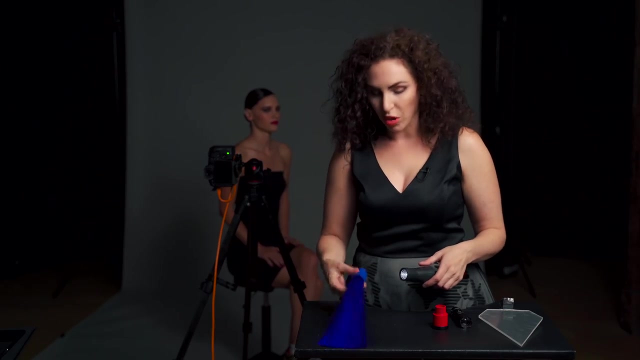 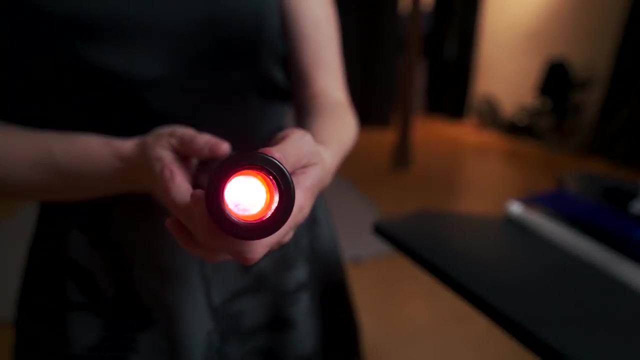 adapter. So basically it attaches in and then on the other side you can actually screw in a variety of different light painting tools. So, for example, you can screw in the fiber optics or a gel or this thing. I haven't played with this one yet, So my goal today is I want to play around. 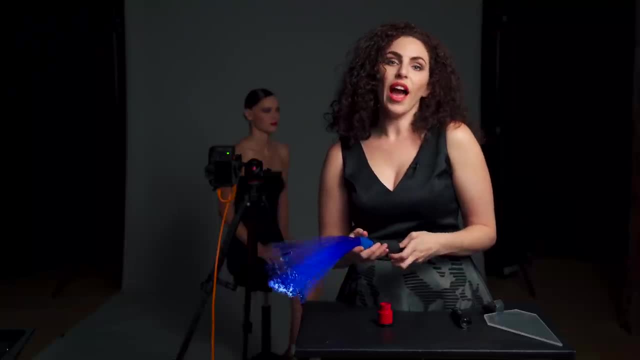 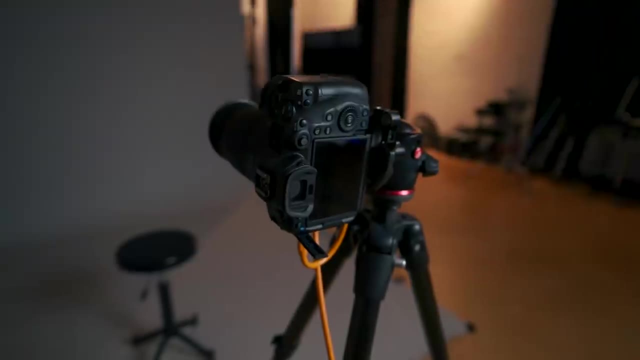 specifically with one of the gels, so changing the color of the light and some of the fiber optics. Now a couple things I know that I need for light painting. I'm going to need a tripod so that I can have really long exposures. I'm thinking this will be at least 10 seconds of exposure, so I need to. 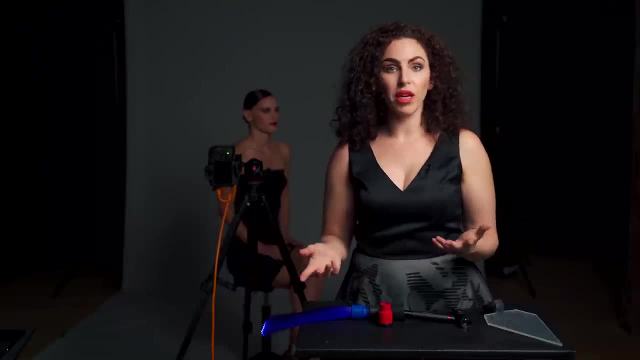 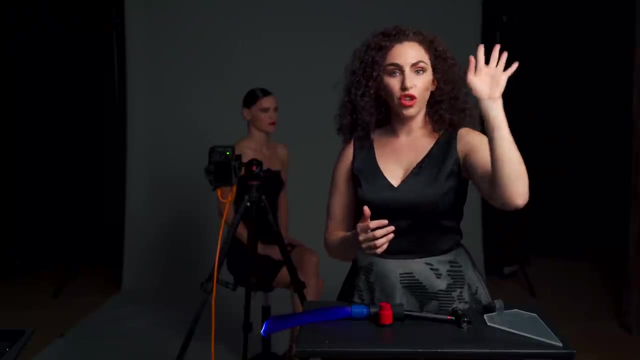 be on a tripod. The next thing that I need is to get rid of ambient light, and I've already done that in this space. I've turned off all of the overhead lights, I've closed the windows and I'll eventually turn off the light that's illuminating me, Because during this long 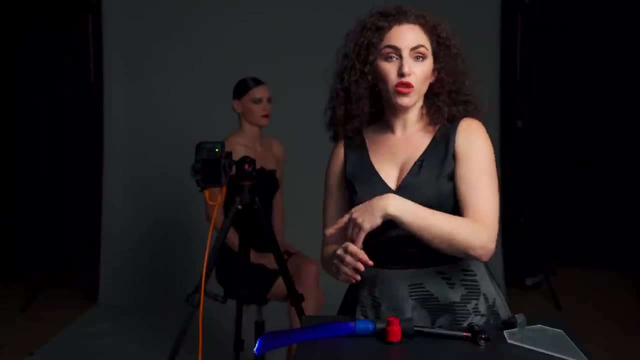 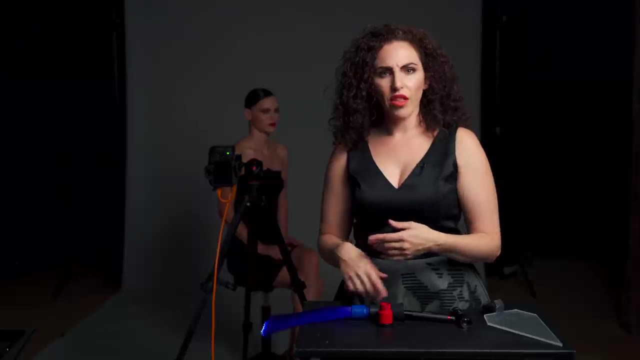 exposure, any light is going to show up, And then I'm also going to need to, of course, shoot on man manual or something to allow me to keep my shutter open for a long time. There's actually something called bulb that when you compress the shutter, it allows the light to expose to. 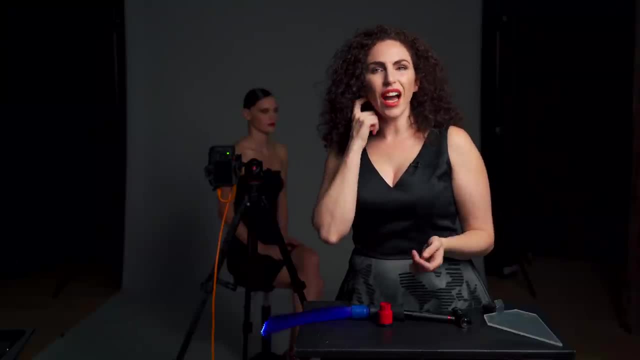 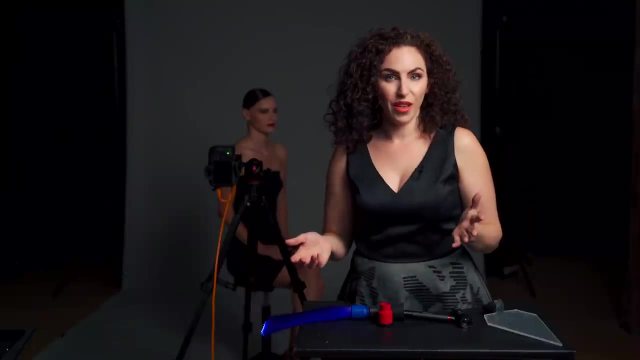 the sensor for as long as you're holding the shutter down. And so in this case, I don't think I'm going to do that, I'm just going to use my tripod and probably- I don't know- 10,, 12,, 15 second exposure Now with these fiber optics. I haven't done this before. 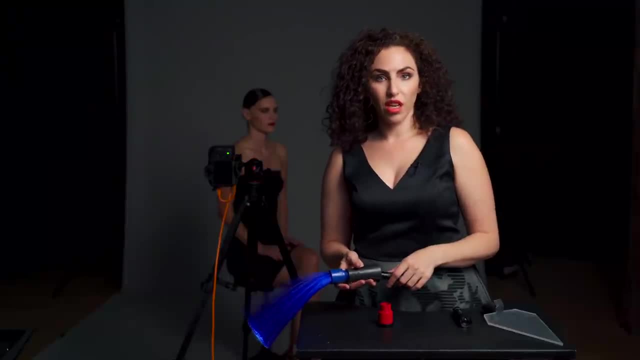 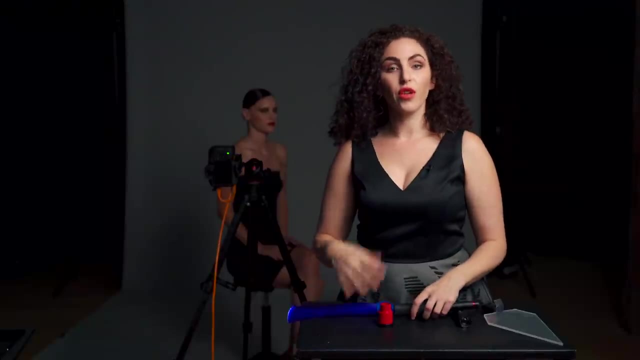 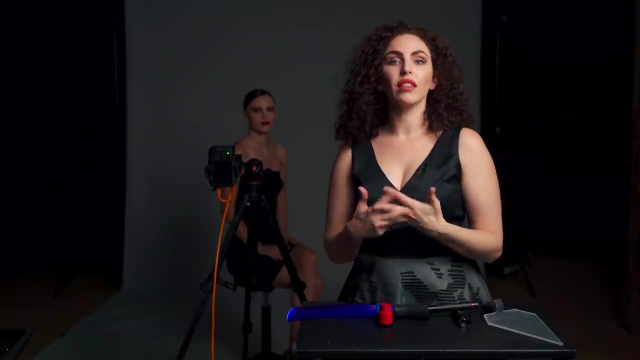 but I've seen some images where they have used this technique. So the idea is is that I'm going to trace it along my subject, maybe along her face or her shoulders, And during that long exposure it'll create streaks of light. I'm also going to have my assistant help me light the background. 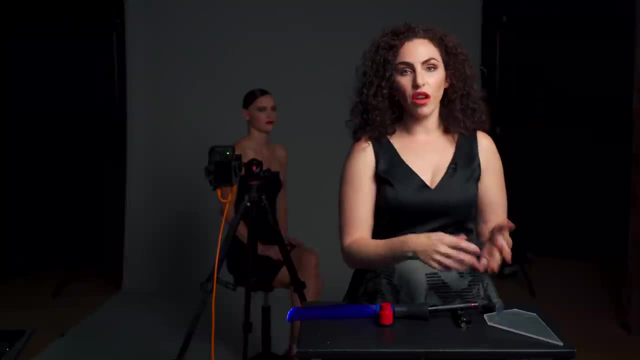 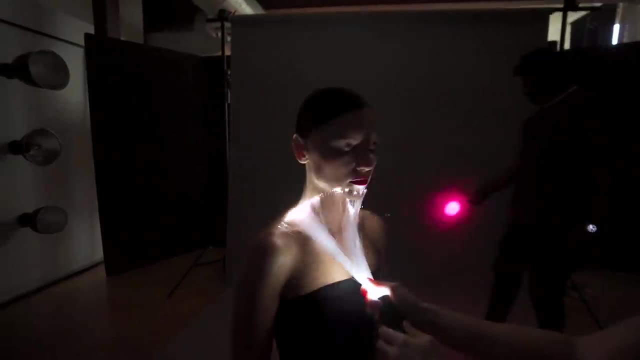 So multiple hands can be doing multiple things. So, for example, we could use another one of these flashlights with a gel and then kick a little bit of light on the background so the subject isn't just blending in there, Maybe another little bit of a dash of color. So my goal is to go in. 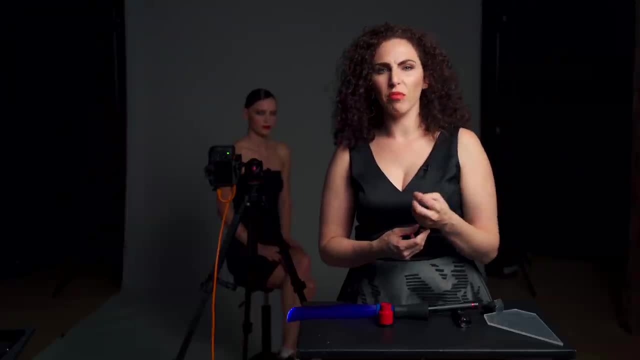 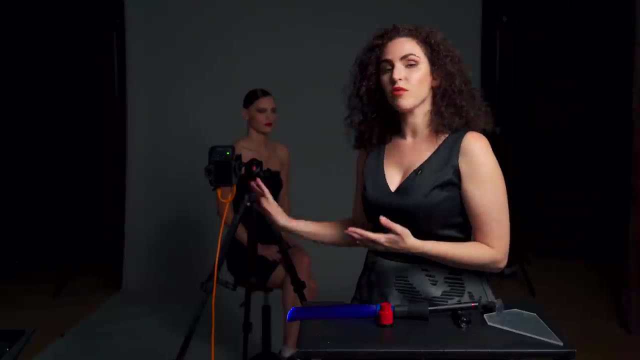 cool tones: blues and reds, Whites and maybe a little bit of like, pinks and purples- and, honestly, just experiment. Now, when I do this, I'm shooting on my tripod. What I'm going to do is I'm going to pre-focus on my model, So